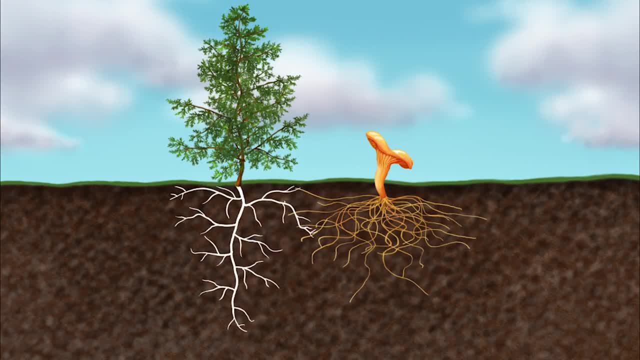 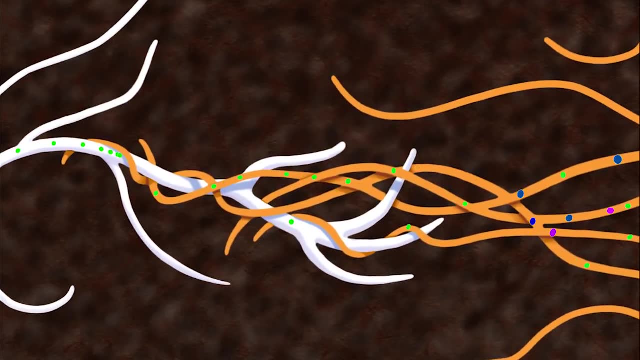 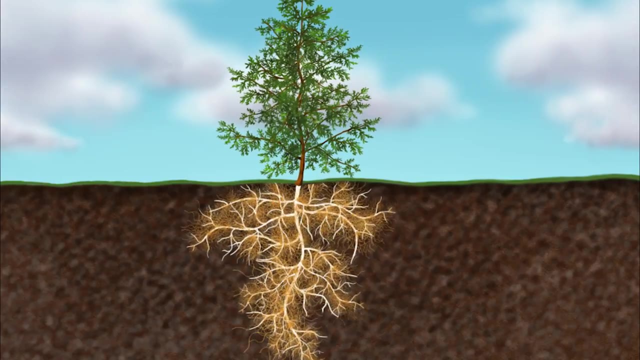 mutually beneficial relationship with each other. The plants give the fungi sugars that they produce through photosynthesis. In exchange, the fungi give the plants nutrients and water that they extract from the soil. Eighty to ninety-five percent of land plants benefit from some type of mycorrhizal relationship. The mycorrhizal fungi are also known as mycorrhizal. fungi. The mycorrhizal fungi are also known as mycorrhizal fungi. The mycorrhizal fungi in some ways are a product of the same species, But not all mycorrhizal fungi have the same. 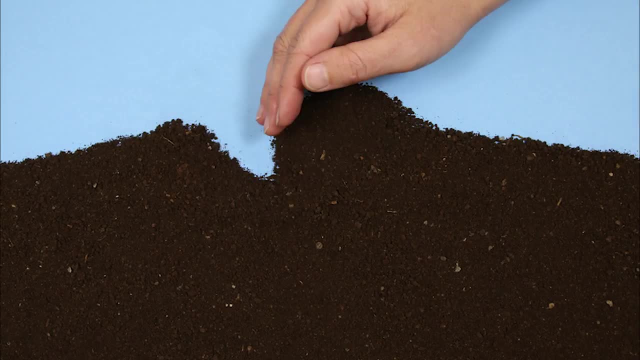 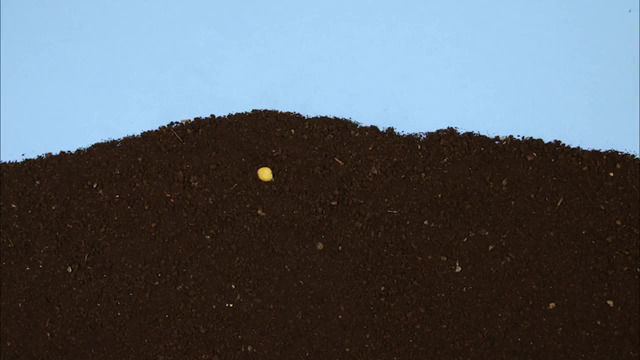 relationship. What does this mean for gardeners? Let's say you plant a seed in soil without any mycorrhizal fungi, The plant's roots will go out in search of nutrients and water to feed its growth. As the available resources are used up in one area, the roots grow further and further. 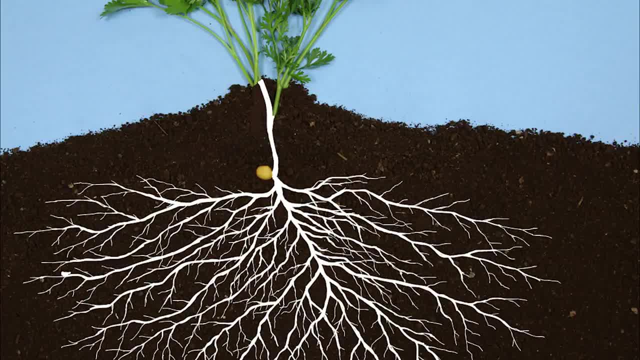 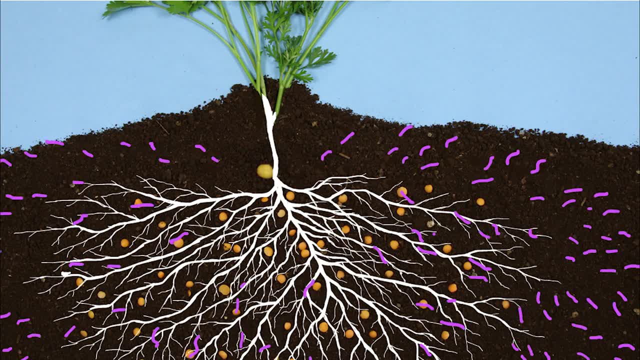 out, expending more and more of the plant's energy. Now let's introduce some mycorrhizal spores. The plant sends signals out to any mycorrhizal fungi in the area and the spores respond by growing hyphae in the direction of the signal. 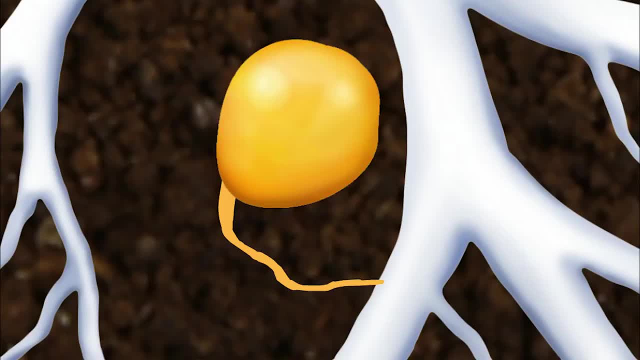 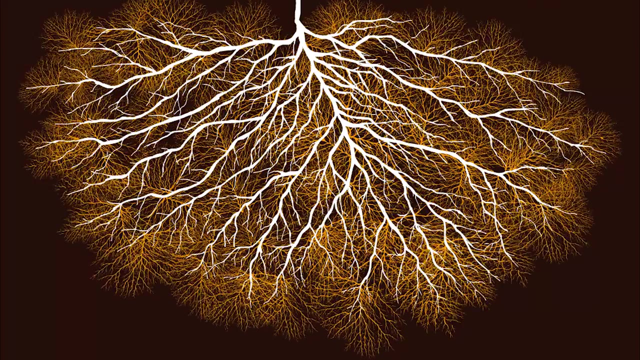 If a spore is able to find the root of the plant, the hyphae will penetrate the root and begin to grow structures that allow for the plant and the fungi to exchange resources. The mycorrhizal fungi will now begin to grow an extensive cotton ball-like mass that will 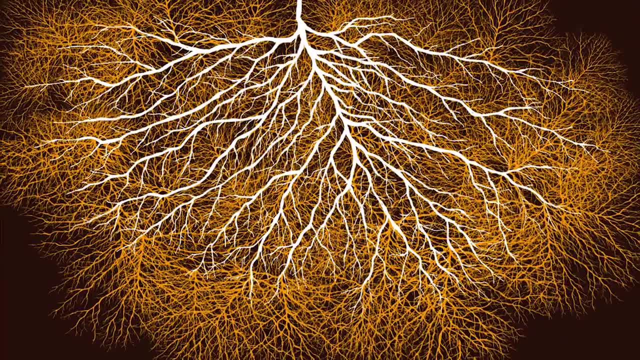 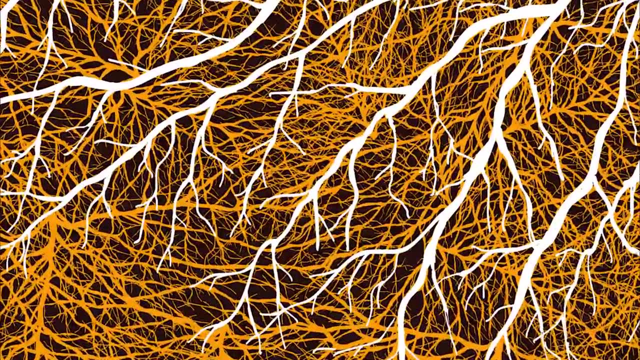 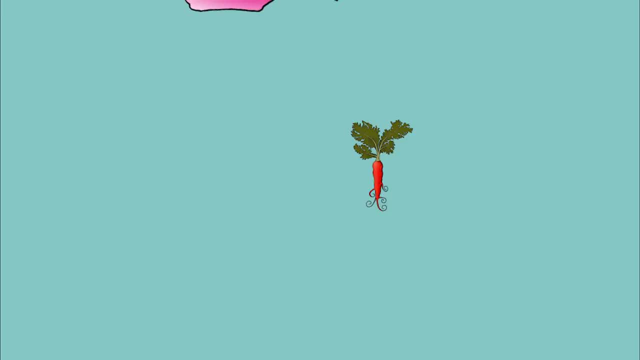 give the plant access not only to the nutrients and water outside the reach of its roots, but since the hyphae are so small, they can access nutrients in the small spaces between the roots as well. Though most commonly grown plants will benefit from mycorrhizal applications, there are a 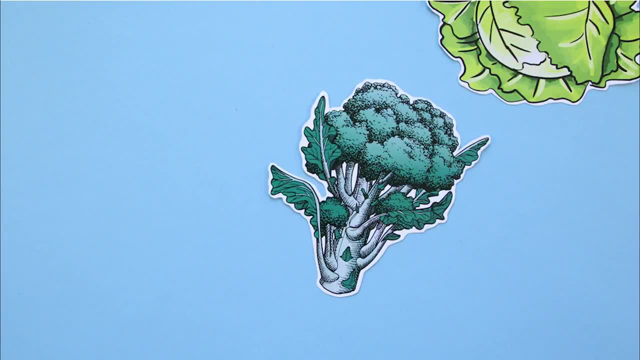 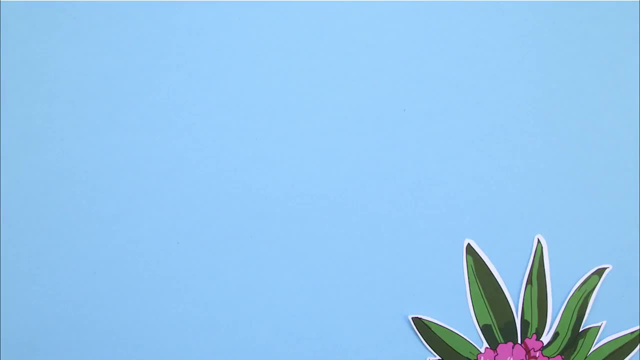 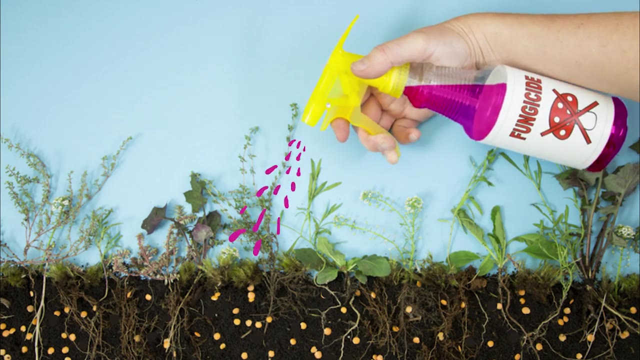 few exceptions. The Brassica family, which includes plants such as broccoli, cabbage, radishes and kale, is one. Beets, chard, blueberries, cranberries and rhododendron are some others. Though mycorrhizal fungi are naturally occurring in most soils, the application of fungicides 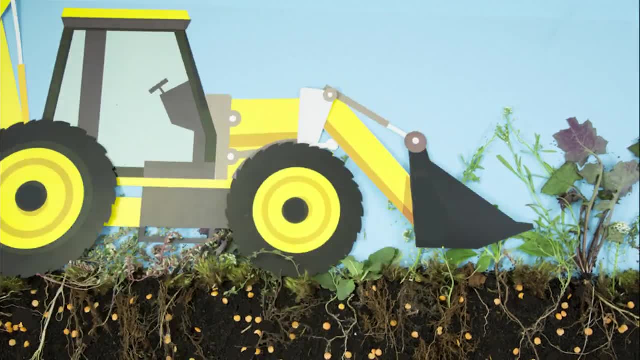 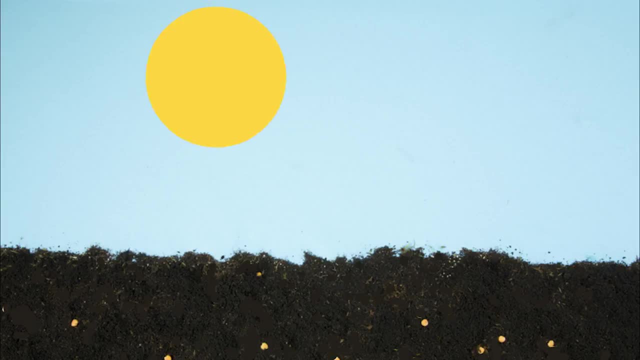 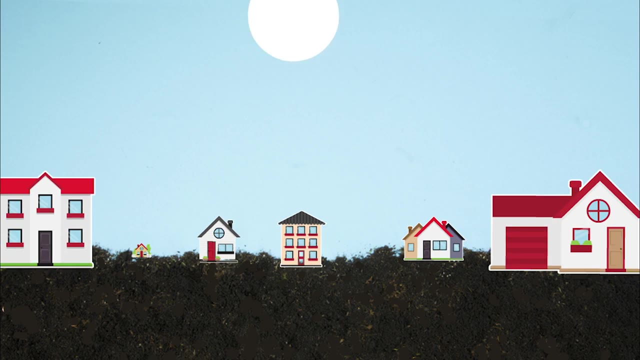 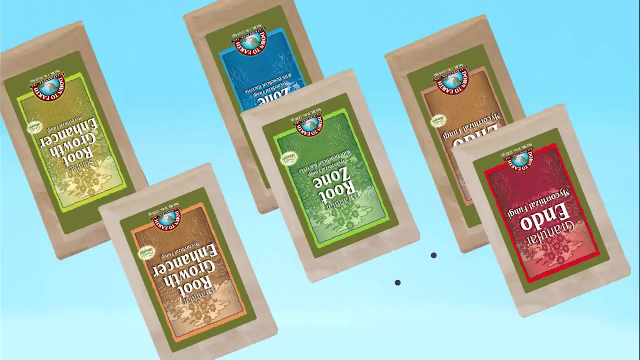 and pesticides. the use of heavy machinery and leaving soils without any plant growth for weeks at a time have created soils with little or no mycorrhizal fungi populations. The ground surrounding newly built residential neighborhoods and commercial properties is particularly lacking. Only in recent years have commercial mixes become available to reintroduce these important organisms back into garden soils.